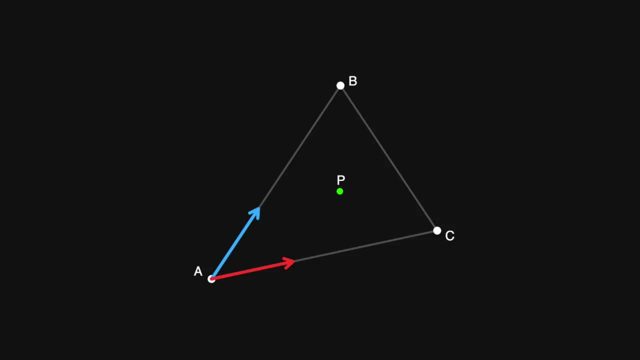 vector pointing from A to C. Together they describe the position of point P relative to point A. Perhaps this is a little clearer if I show the red vector starting from the end of the blue vector. Now, the length of the blue vector is controlled by a weight variable called w1,. 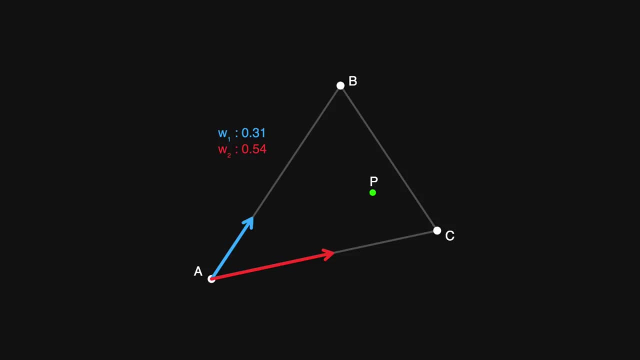 and the length of the red vector is controlled by w2.. When both of these values are zero, that means that point P is at A. If I move point P over to B, then you'll see that point A is at B, w1 is equal to 1, and w2 is equal to 0.. If I move point P over to point C, 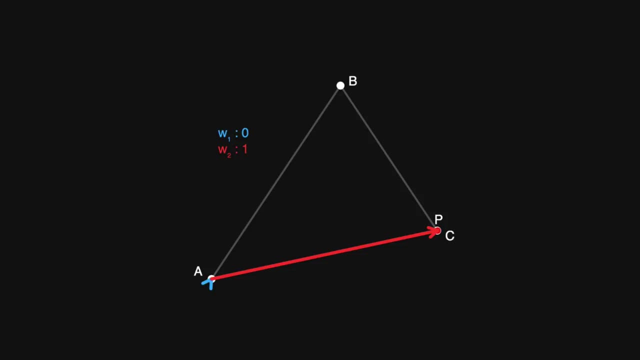 this will, of course, be the other way around. Okay, so this is an interesting way of describing the position of point P, but how does it help us with our task? Well, notice that if I move the point out past the edge AC, then w1 becomes negative. If I move the point out the other side, then w2 becomes negative. 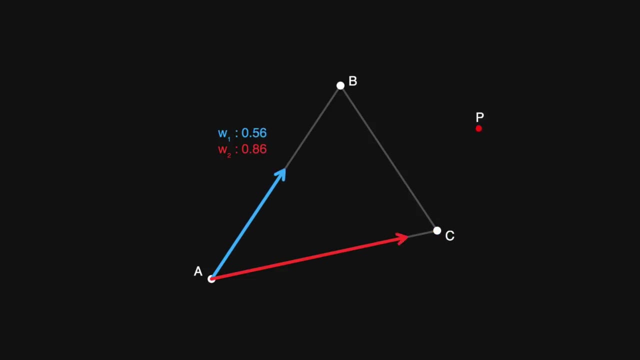 and if I move the point out past edge BC, then w1 plus w2 will add up to be greater than 1.. So if we can figure out the values for w1 and w2, we have a very easy way of determining whether or 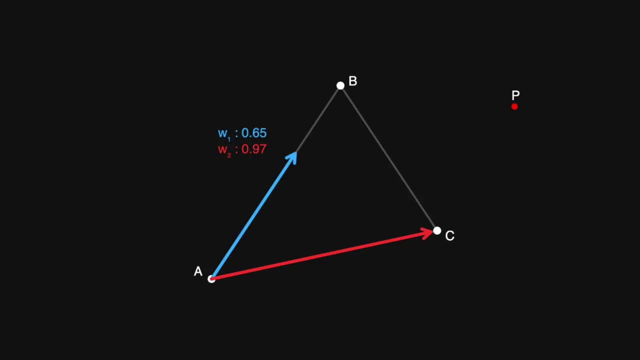 not. P is inside the triangle. Let's write an equation for the coordinates of point P So we can say: P is equal to A plus w1 multiplied by B minus A, plus w2 multiplied by C minus A. So this is just a mathematical representation of what we saw in the diagram. 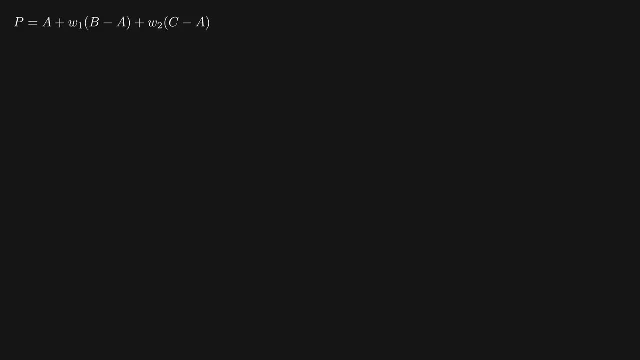 I'm now going to write this equation out again twice, once for the x-axis and once for the y-axis. I'll then rearrange the second equation to get w2 isolated on the left. We can then easily take this expression for w2 and substitute it into the first equation to get a new equation. 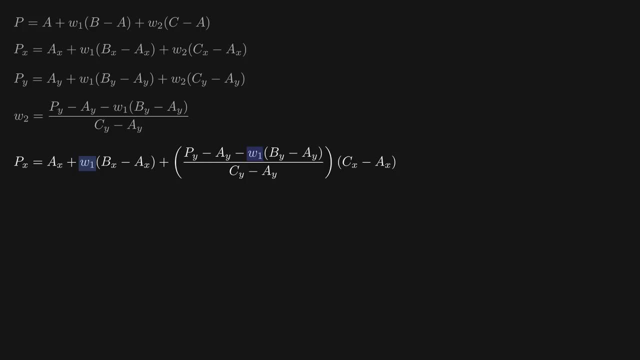 with only one unknown, w1.. Our task now is to isolate w1 on the left side of this equation. This should be fairly straightforward algebra, although, of course, having this many variables, it is quite easy to make a mistake. So let's work through this methodically.